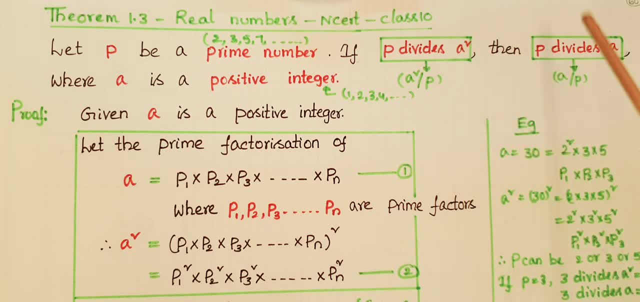 divisible by the that prime number. So here we have to prove that p divides a means a is exactly divisible by p. So here, given a is a positive integer. so we know that as per fundamental theorem of arithmetic any composite number we can express as product of the prime factors. So 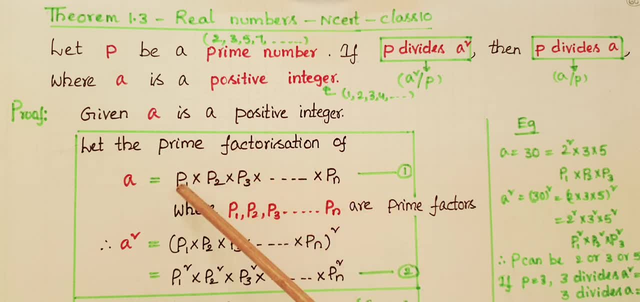 here a we can express as product of the prime factors, that is, p1 into p2, into p3, into, etc. into pn. This is first equation here: p1, p2, p3, etc. pn are prime factors and squaring on both sides then a square is equal to p1 into p2, into p3, into, etc. into pn. whole square that is equal to 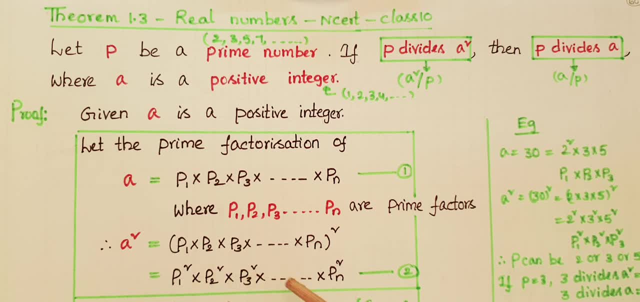 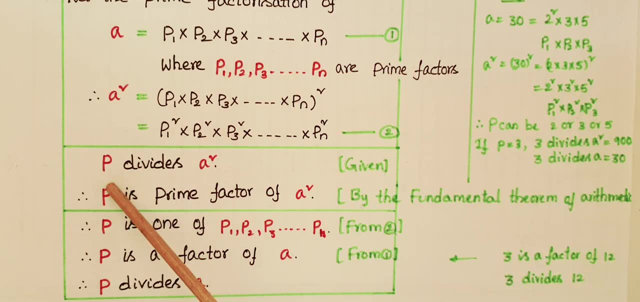 p1 square. So this is second equation. Now the given statement is: p divides a square. that means a square is exactly divisible by p or p is a prime factor of a square. From second equation: a square prime factors are p1, p2, p3, etc. pn. But here p is a prime factor of a square, so p is one of these prime. 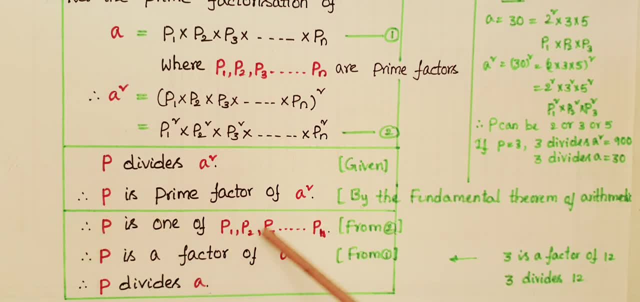 factors. Therefore p is one of these prime factors: p1, p2, p3, etc. pn. So here p is a prime factor of a square. so p is one of these prime factors: p1, p2, p3, etc, pn. So if p is a factor of a means p divides a. 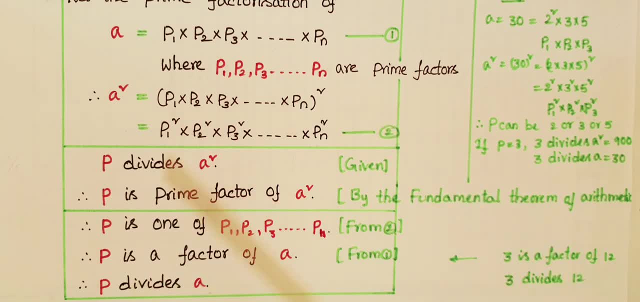 from second equation, and here p1, p2, p3, etc. pn are already prime factors of a. Therefore p is also a factor of a, so p divides a. If p is a factor of a, means p divides a, or a is exactly divisible by p. 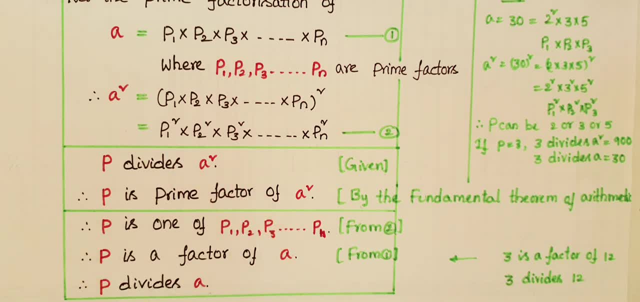 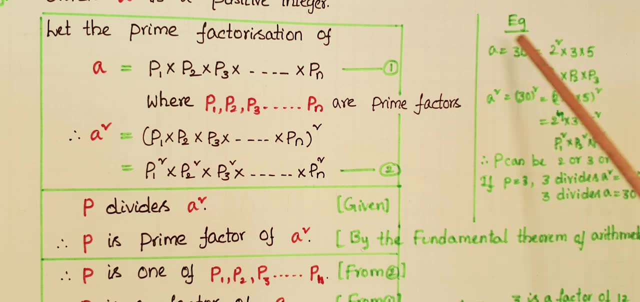 Therefore, if p divides a square, then p divides a. Now you can see with an example. for example, let the positive integer a is equal to 30, so you can express this positive integer as product of the prime factors. so we can express 30 as 2 square into 3, into 5. so here the prime. 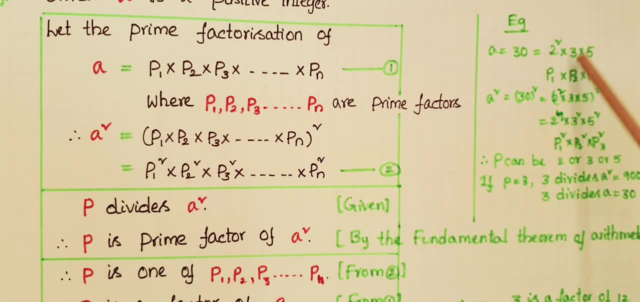 factors are 2, 3, 5, p 1, p, 2, p, 3 are 2, 3, 5. so a square is equal to 30 whole square, that is equal to the prime factors whole square. so 2 square into 3, into 5 whole square, that is 2 to the power of.